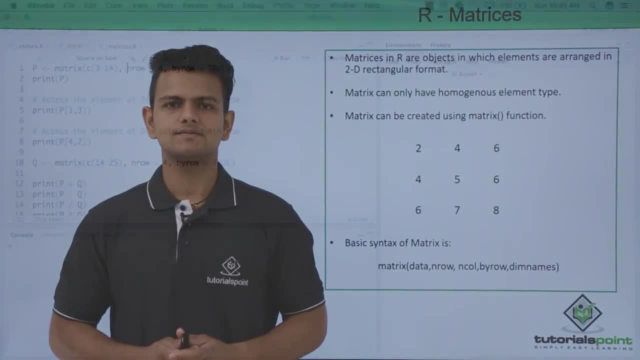 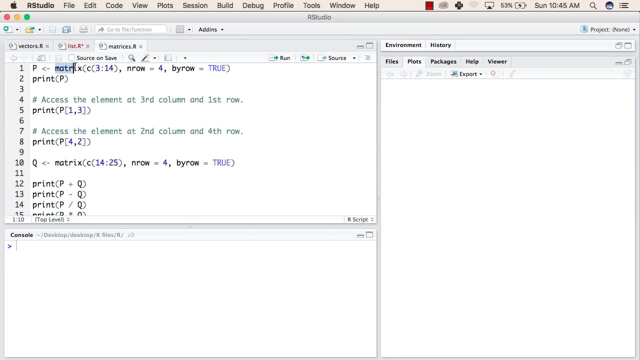 see how we can implement matrices in R. In the first line, we have created a matrix with the name p. We have used metric function to create the matrix and the values inside this matrix will be from 3 to 14.. The number of rows will be 4 and this will be aligned. 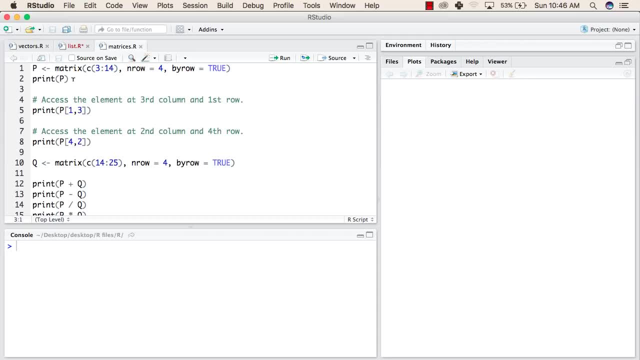 by rows because by row is true. Now we'll try to print our matrix and create this. So the values inside this matrix are 3,, 4,, 5, from 3 to 14.. This is aligned by row. If we made by row false, then the values would have been aligned by columns. 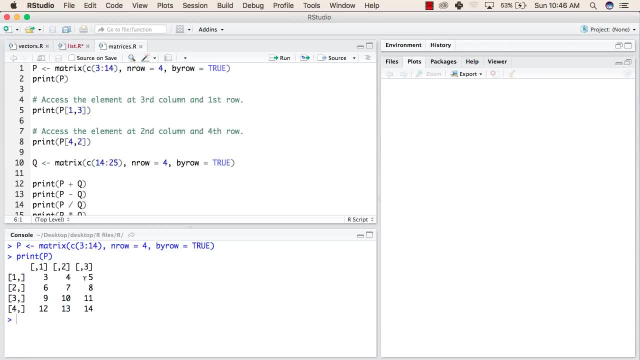 Now we'll try to access the element at third column, that is, this column and first row. That is when we try to access this element. this should be 5.. When we select by dragging, then keep in mind that you drag. 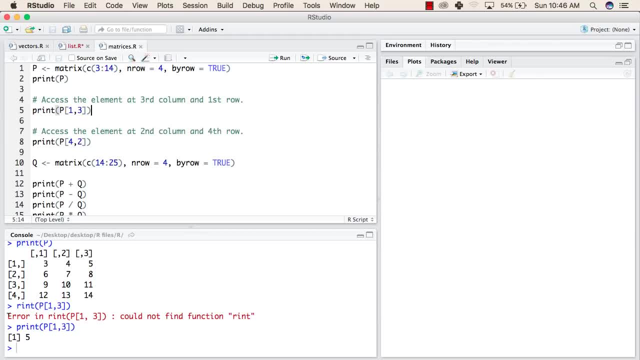 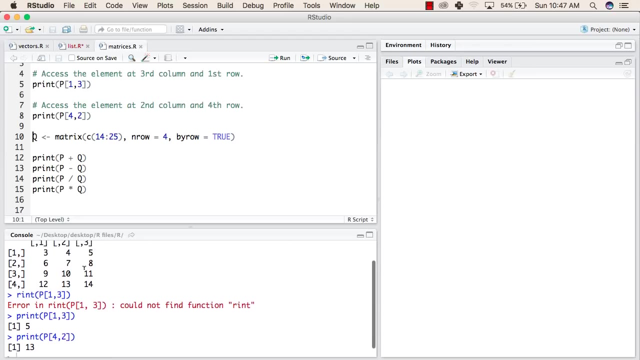 the complete line. Otherwise, this will show an error like this, because we did not select p and we selected this much line, So this gave us an error. Now we'll try to access the element at second column and fourth row. This should give us 13 as the second column and fourth row. 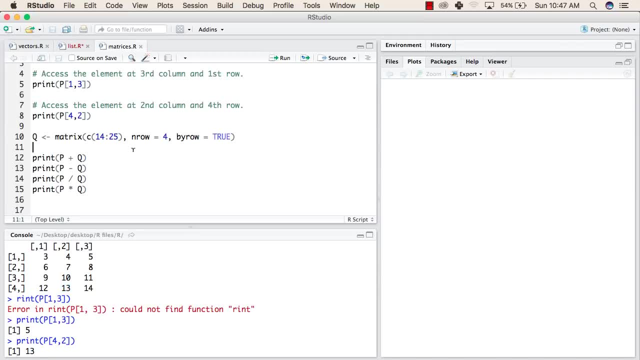 So this element. Now we'll try to make one more matrix, Q, with values 14 to 25, same as the previous values, same as the previous matrix. It will also have four rows that are aligned by row. Now we'll create this matrix and now we'll try to perform. 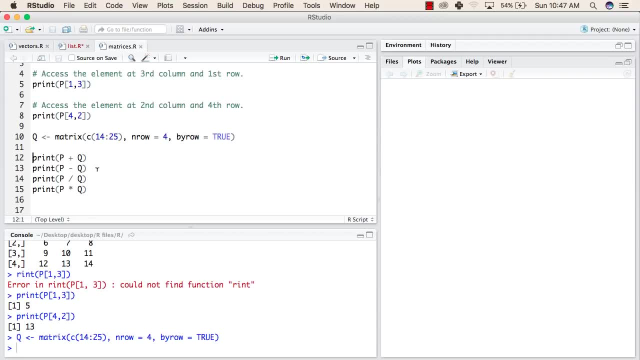 some mathematical operations on these two matrix. First will be addition of p matrix and Q matrix. This should give us the sum of first matrix and the second matrix. Similarly we'll perform subtraction of first and second matrix And similarly we'll perform division and multiplication also. 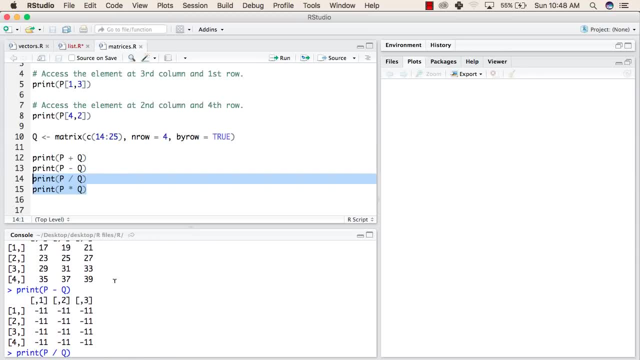 So these are the mathematical operations that you can perform on matrix. Thank you.